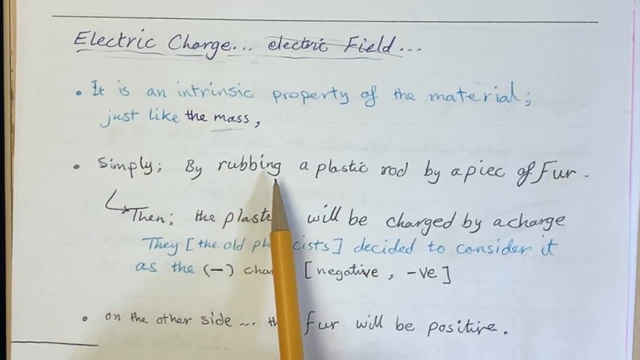 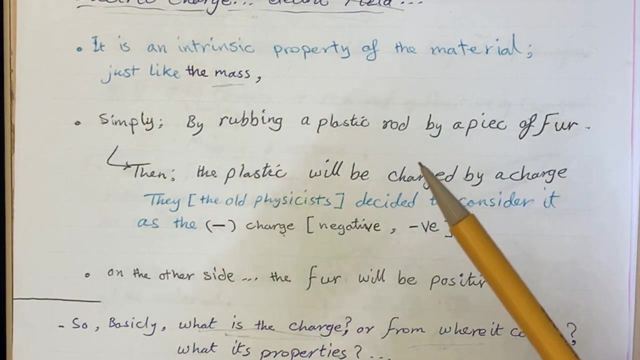 if we, for example, rub some plastic piece or rod with a piece of wood, then one of them will be negatively charged and the other will be positively charged. And using this rod with some small pieces of paper, it will attract them and it will show us that this rod is charged. 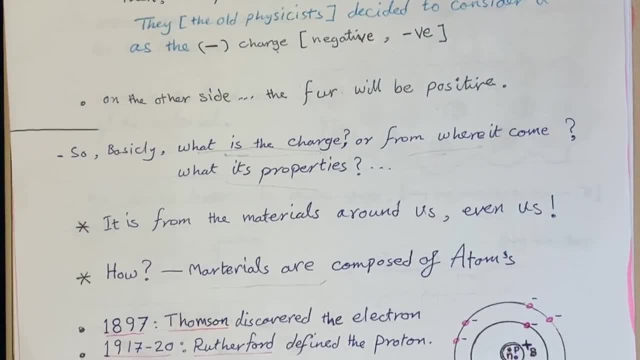 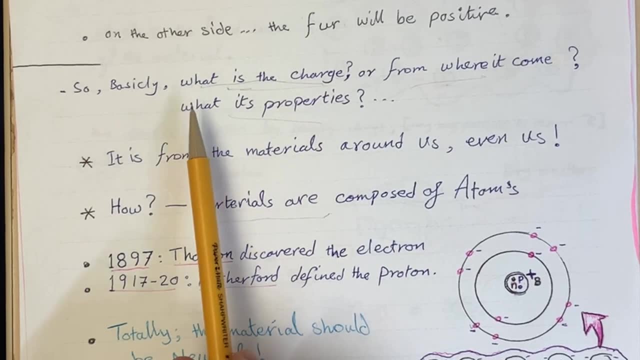 Now, basically, what is the charge? From where does the charge come And what are the properties of that charge? After understanding these questions and their answers, then we will be done with this lesson today And we will start to understand what we need to apply using this quantity in physics. 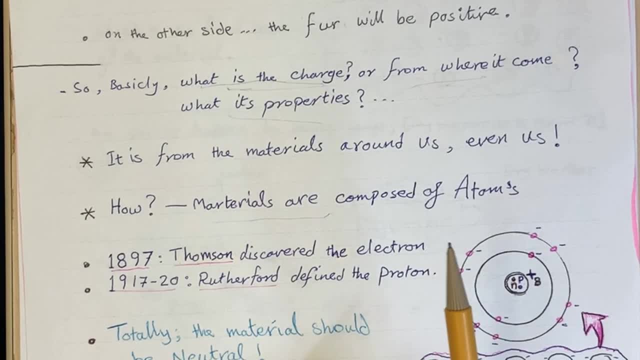 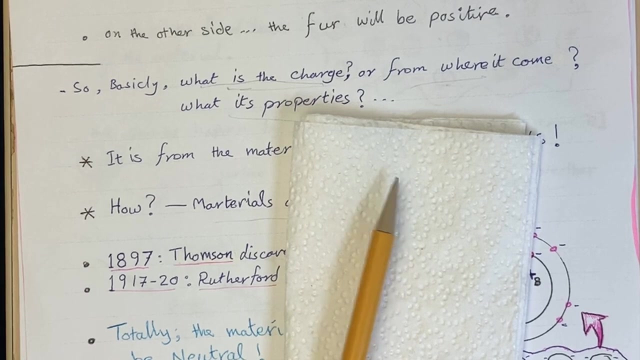 Actually the previous physicists in classical physics. they decided and they found actually that the charge came from objects, from the matter. For example, if we have a plastic piece and a four piece and we do this experiment, then one of them will be charged by negative, the other by positive. 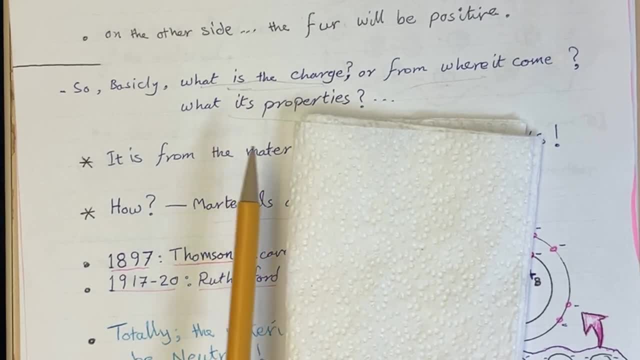 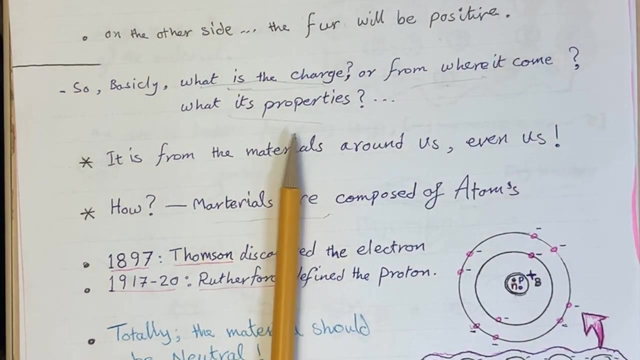 We won't know enough about positive and negative yet, but the charge came from them. It didn't came from outside this system, this closed system, which is the piece of plastic piece of four. okay, So that charge came from the material. 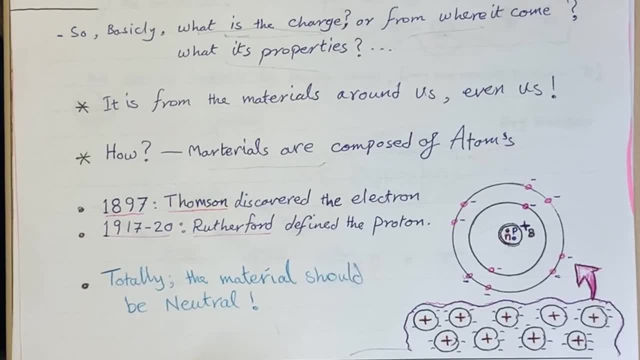 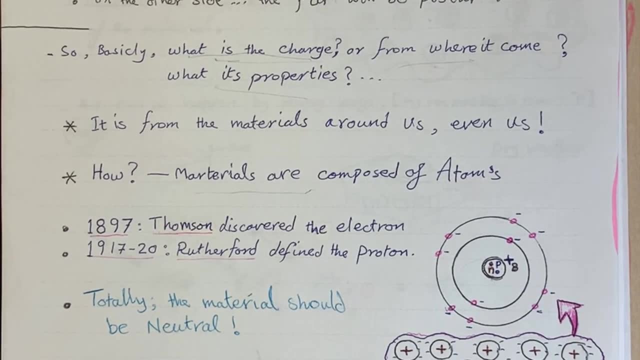 Let us remember the construction of any material. We know that the material is composed of atoms or molecules. Let us talk about atoms. This is the simple model for the atom. It's a nucleus with electrons rotating around that nucleus And there's some neutral neutrons inside the nucleus. 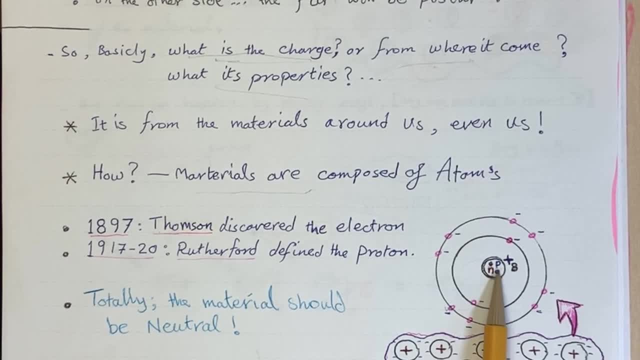 And some positive protons inside that nucleus too, And there are many electrons rotating around this nucleus in orbitals, And the number of these negative electrons is the same as the number of the positive protons inside that nucleus. The nucleus is fixed in itself. 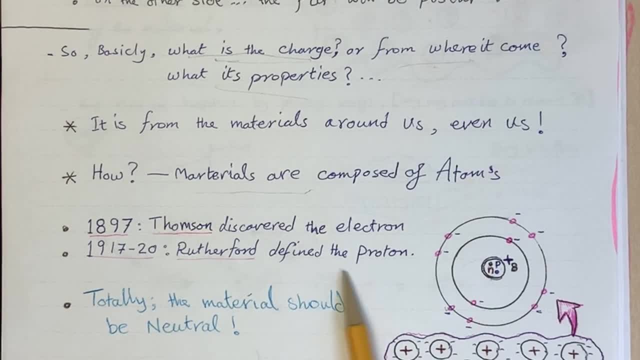 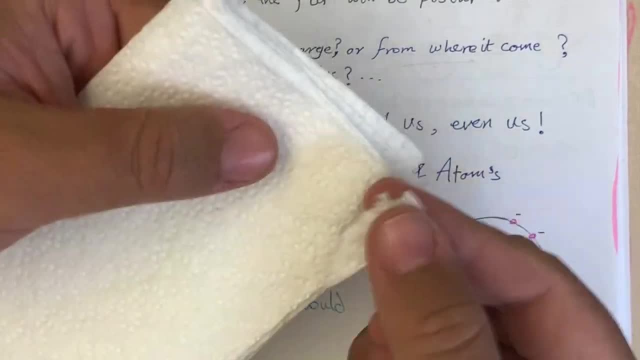 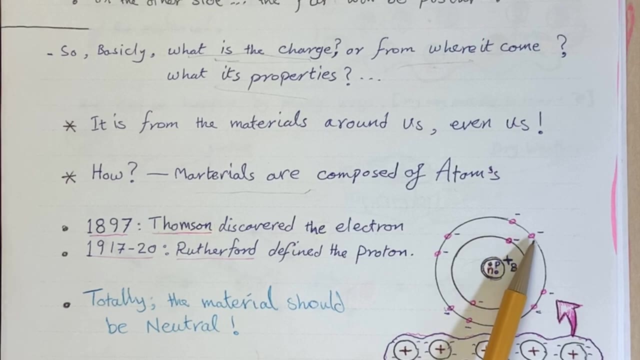 It's a place. We cannot move a nucleus from its place. Just, we can do that by dividing the material. We just divide the material, then that we are moving nuclei from one place to another and separate them, But the electrons, they are already moving. 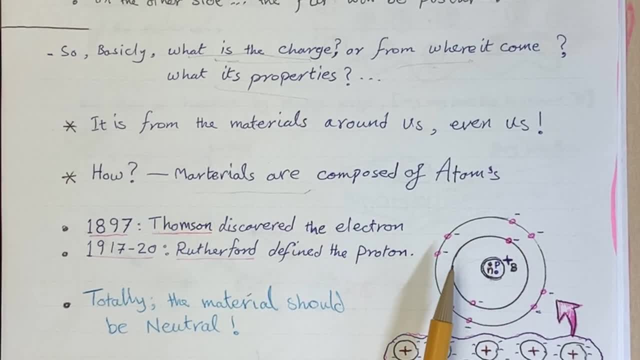 So we can study them easily. We will see that now. So the electrons they define and discovered by Thomson in 1897. And the proton was found before 1970 or 2020.. It was found in the 80s, late 80s. 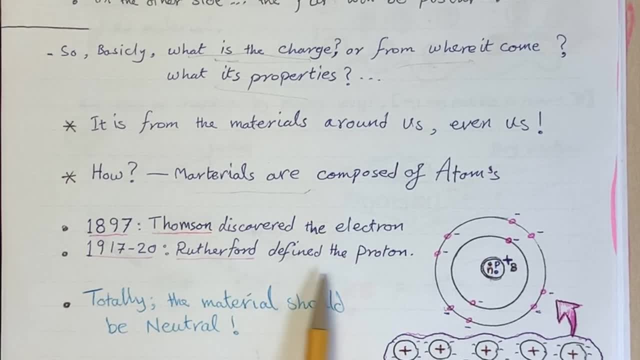 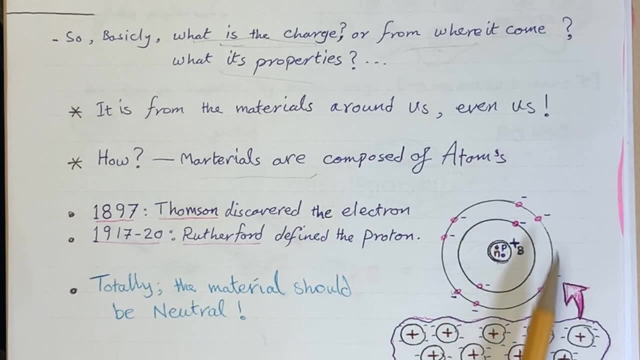 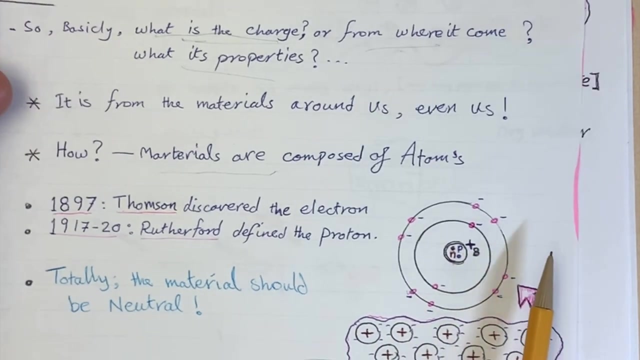 But who defined that this particle is a proton is Rutherford, But totally the material in general should be neutral And there is no charge for any material. For example, this atom is atom, It is not an ion, So it is neutral and it has no charge. 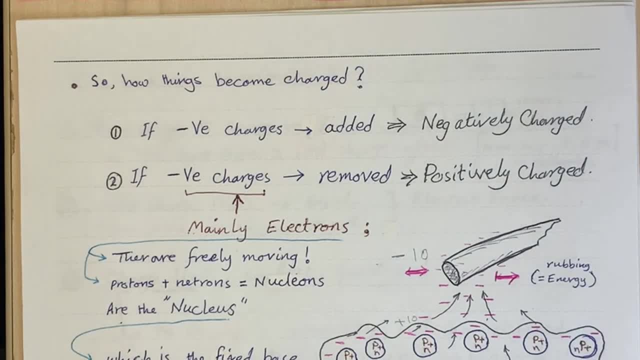 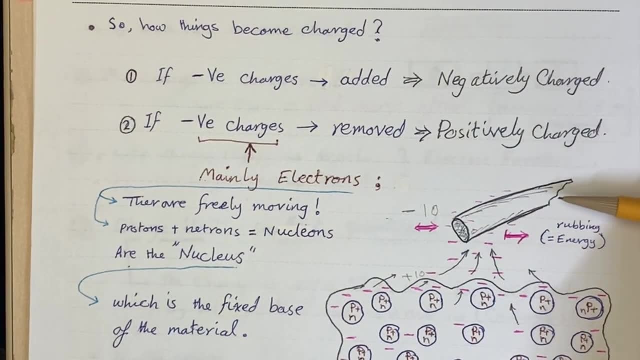 Okay, next, How the things become charged. We have a simple experiment By using a rod of plastic with a piece of foil. If we we are rubbing them, it is not just rubbing, It is actually. there is energy between. 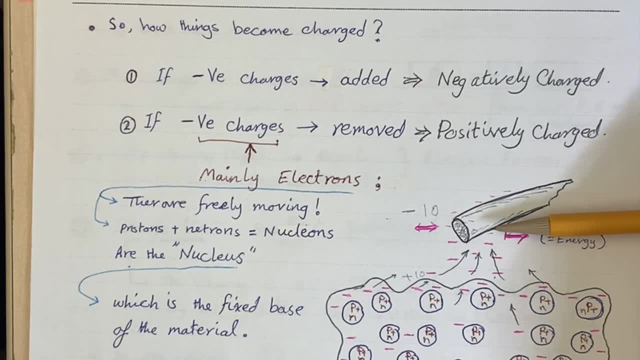 spent here And there is a work done, So this energy is gained between these two pieces of matter. The energy means movement, And this movement is available just for the electrons between these two materials. Some materials tend to lost electrons According to their molecular structure. 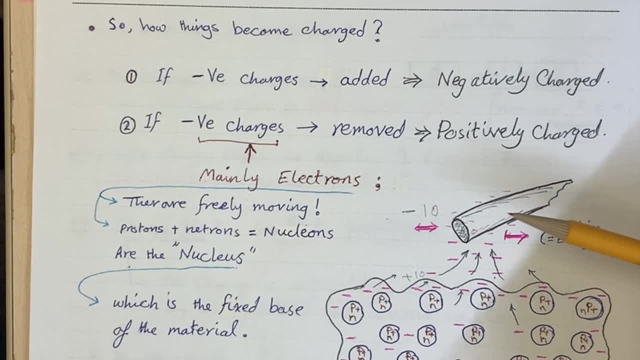 Some material tend to gain or to attract these electrons, So this material will be negatively charged, And the other materials, which are which like to lost electrons, will became positively charged. Actually, during this interaction, energy will be transferred from body to another. 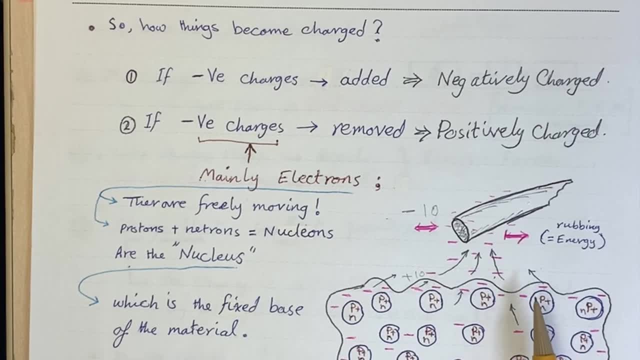 And the most likely particles like to gain this energy is the electrons, And these electrons will be easily freed from the surface of one material to go to another material. In this case, and we will see how this will happen- In this case, one material will be positively charged. 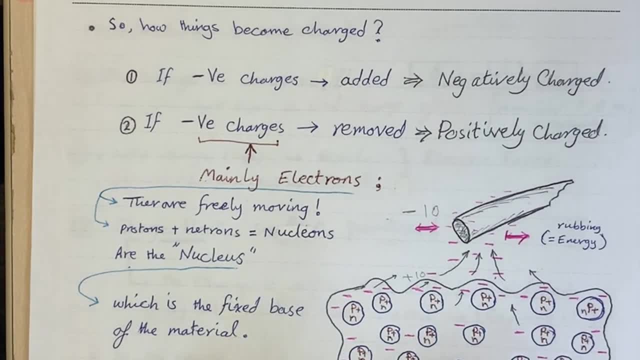 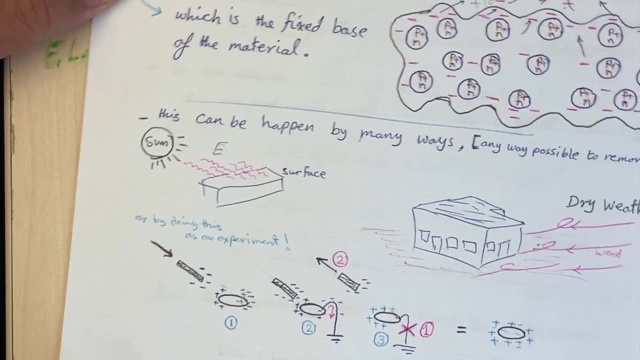 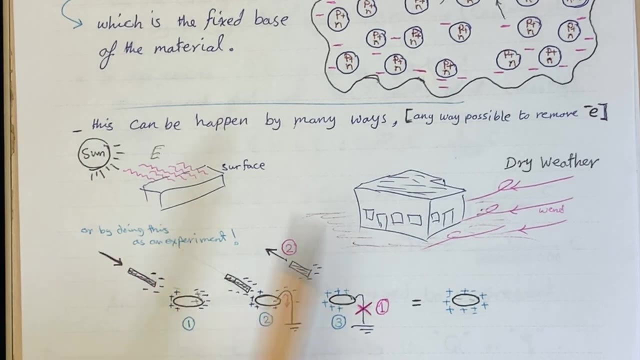 and the other is negatively charged, But the nuclei again will stay in their places As another, as other. some other examples how material will be charged, For example, if we have a plastic surface and the sun attack it- the sun rays or photons. 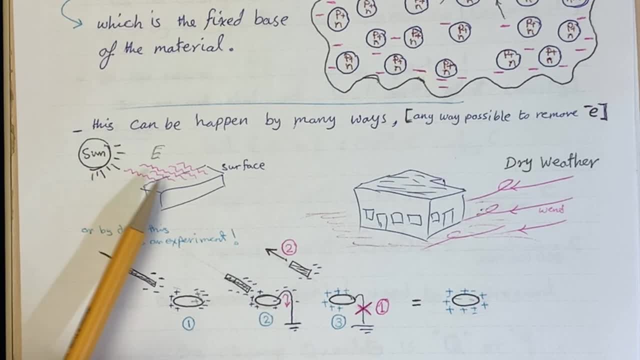 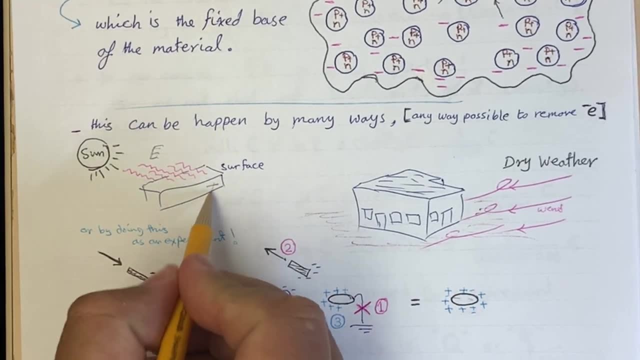 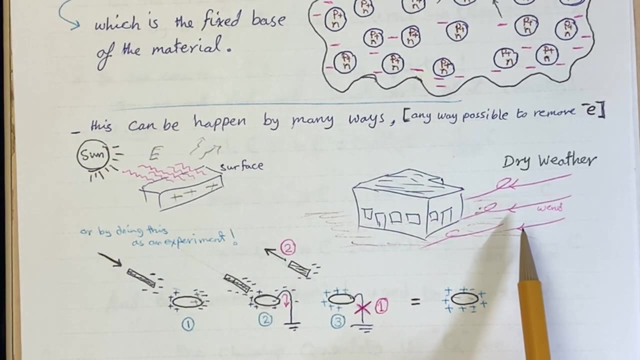 will transfer some energy to the electrons and allow these electrons to escape from this surface and leave this surface positively charged and the electrons go with the wind. Okay, Some other example, which is we see it always If we have in dry days and we have dry wind. 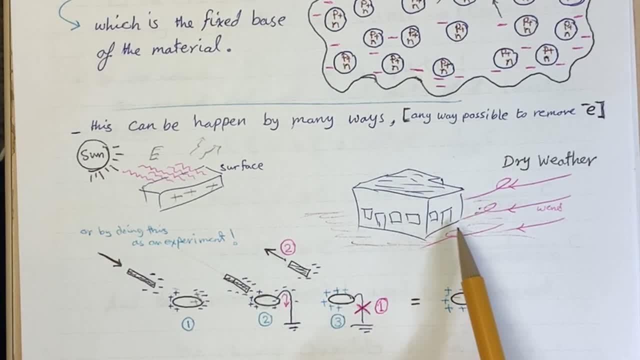 this wind is robbing or attracted. interaction interacted. This wind interacted and robbing with the bodies like the house or the furniture inside the house and make this, this body or that charged. When we interact with this body, we can see some sparks. 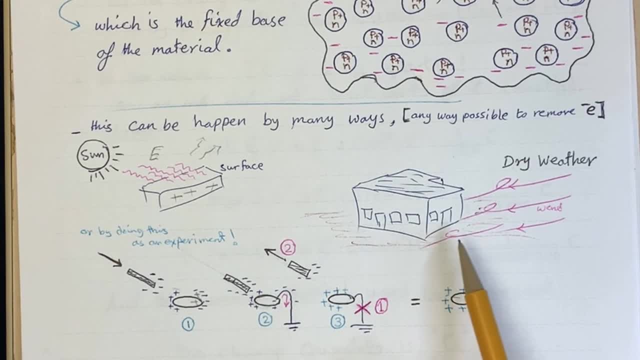 or some annoying feeling by discharging. You know that I believe that- Or we can do this professionally by doing an experiment which is a simple experiment, By closing a rod with which is charged rod to a piece of metal, for example. 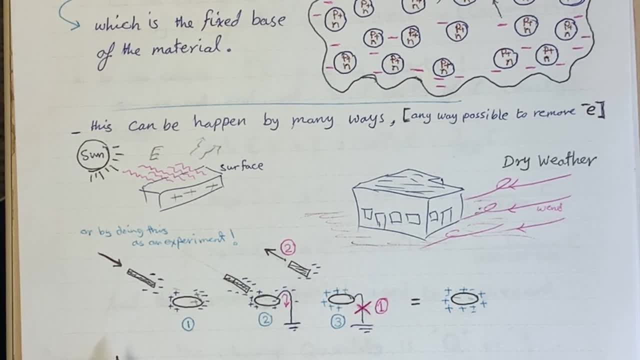 we can object here. If this is, if this rod is charged by negative charge, then it will repel the negative charge. make them go away from this closed side. make the positive charge in the closed side and the negative charge in the far side. 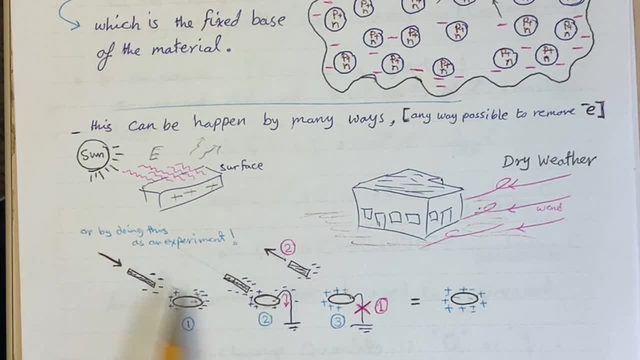 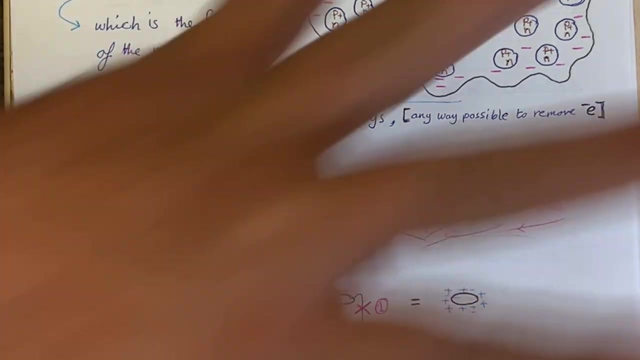 And simply, if we remove this first object, then the negative charge will go back and the object, the second object, will still also neutral, without charge, without charging. Now, what we, if we need to make it permanently, permanently charged? Now, if we need to make it permanently charged. 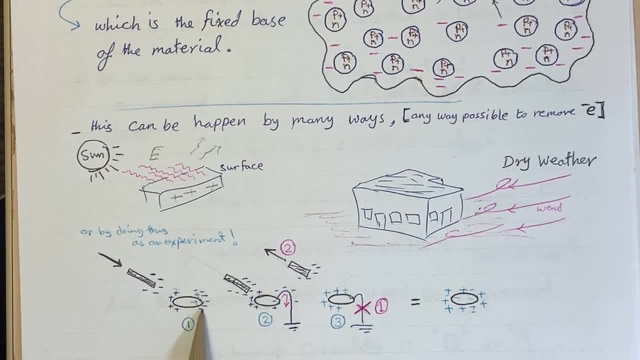 we need to let those negative charge, for example, free to be escaped from that side by grounding. By grounding now this these charge negative charge will escape to the ground Again. if we make this negative charge go away, then the negative charge will return back from the ground. 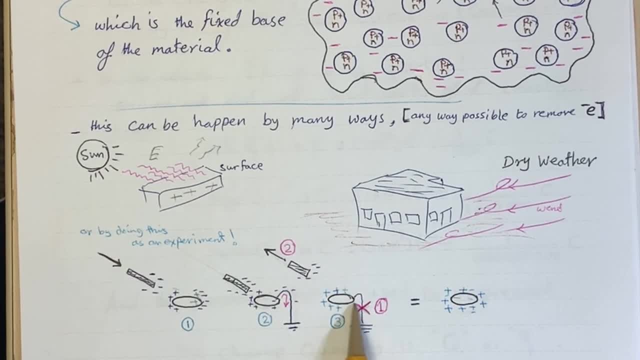 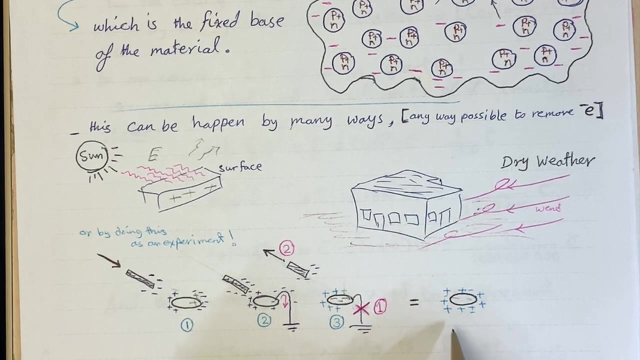 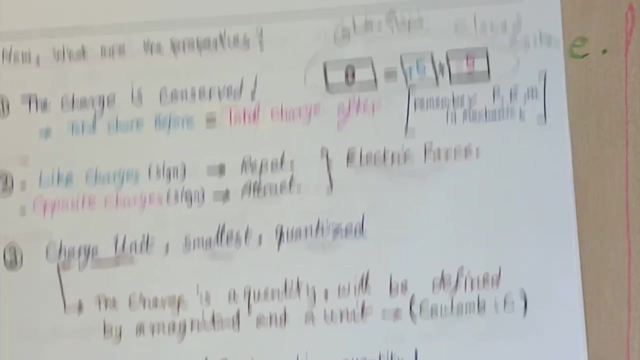 But what we need to do is cut the grounding at first, then removing the affected negatively charged rod. In this case we have more positive charge on the second object with less negative charge on it. Leave it positively charged Means that we have positive charge more than the negative ones. 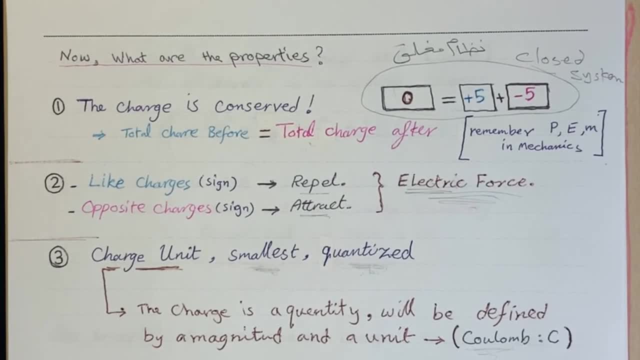 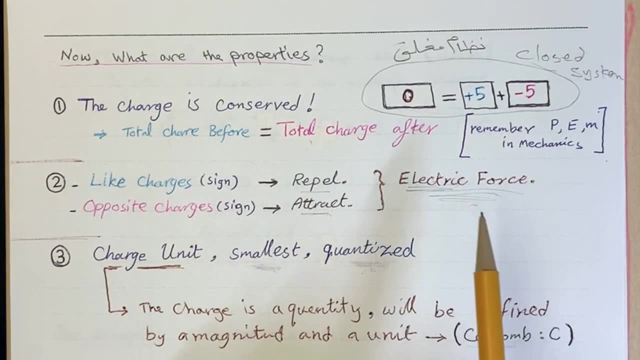 Now we need to focus on the properties of the charge, The charge. we have an important law in physics, or nature in general, which is the conservation of things: Conservation of momentum, energy mass, and so on. Conservation of the charge. 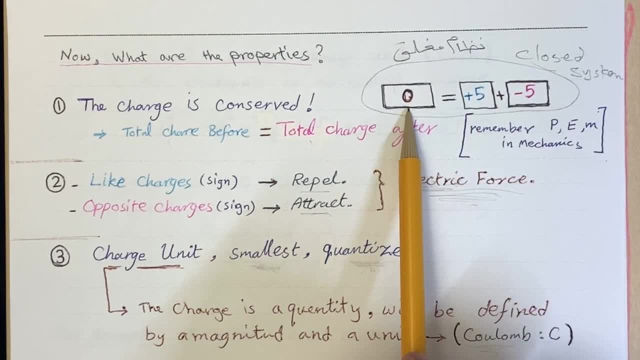 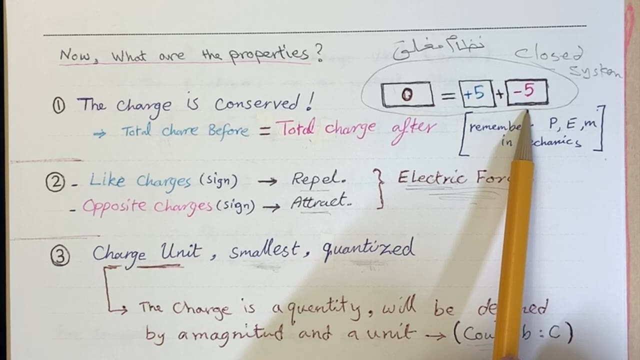 If we have an enclosed system and we have an object and this object with zero charge, which is neutral, if we need to charge it by positive five units of charge, then there should be another object with the negative charge with the same magnitude. 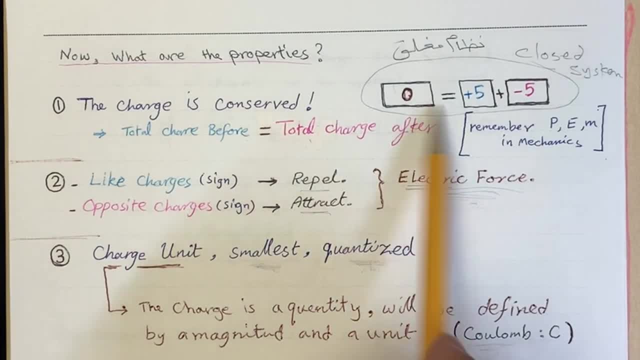 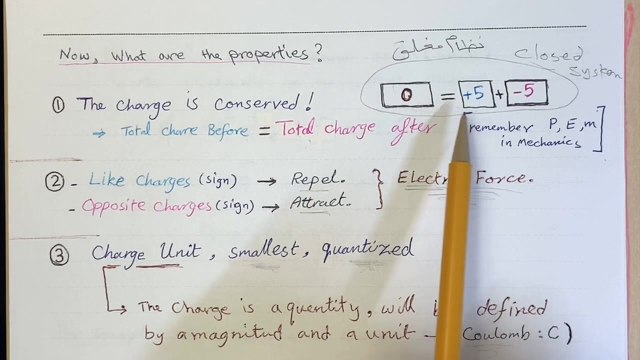 So the total charge before in that system should be equal to the total charge after. So we cannot create new charge or decay a charge. So this is a closed system and the charge should be closed, should be conserved in that closed system. 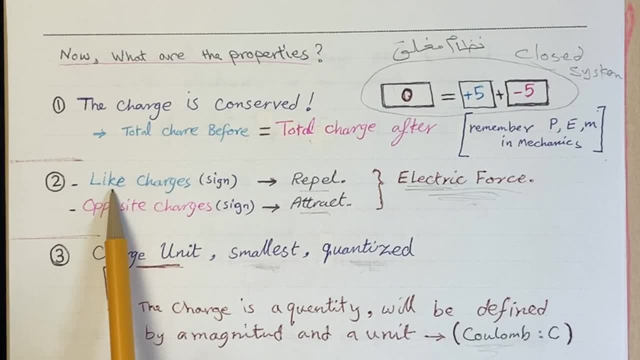 Also another thing. we have the live charge. their signs are repelling each other, But the opposite charge are attracting each other. This is electric force, Electric force. it's an important principle to understand that we have more than one force in nature. 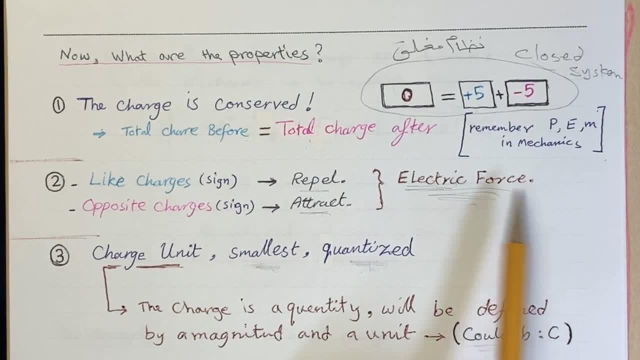 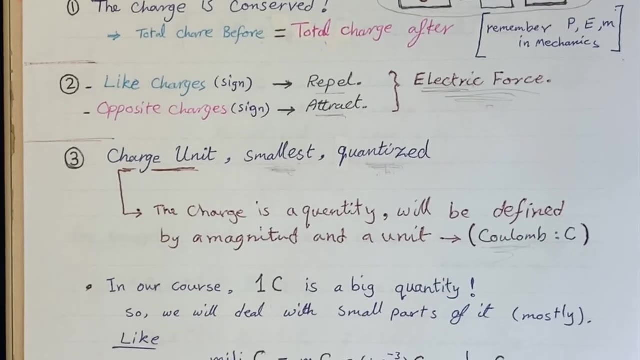 We have magnetic force, we have nuclear force, we have gravitational force and we have electric force. We need to study this force, its properties and how we can apply this force. We will do that in this course. Now, what is the charge unit? 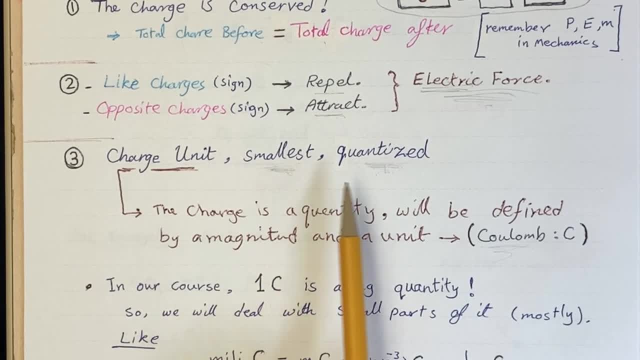 What is the smallest charge available? Also what we mean by the quantization of the charge. So why the charge is quantized? Now, the charge is quantity in physics, and every quantity in physics should be defined by a magnitude, which is a number. 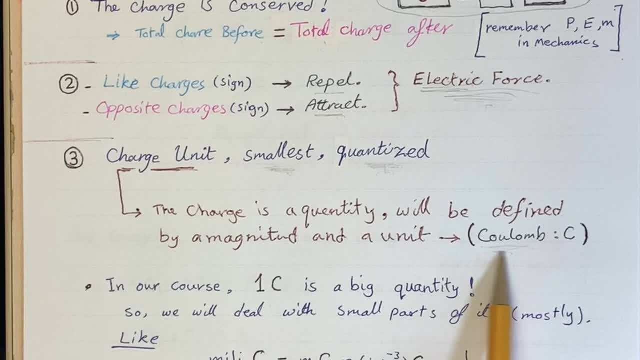 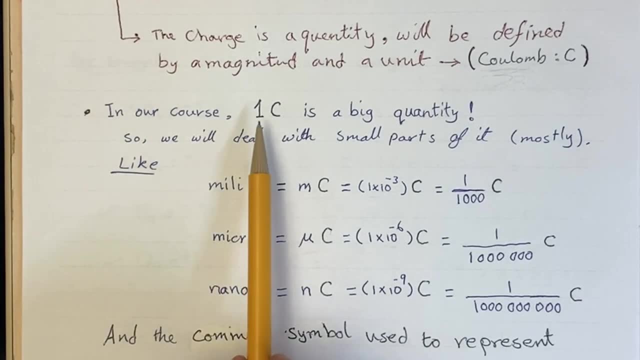 and a unit, and the unit is Coulomb, after the scientist Coulomb. Also, it's important to notice that one Coulomb is a big quantity, For example, one Newton. one Newton is a force which is a sensible force for us. 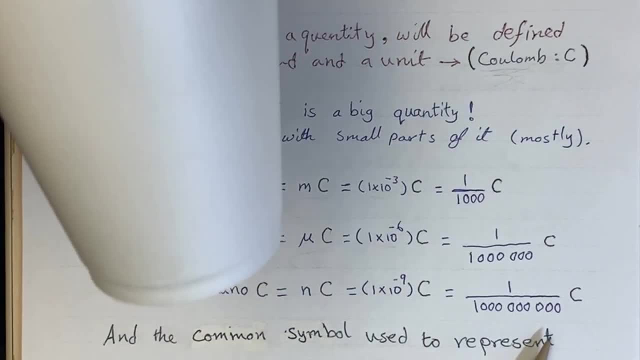 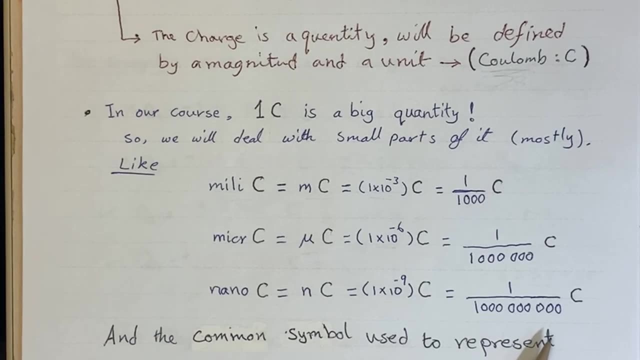 For example, the water filling this cup, which is 100 milligram weight. the force of its weight is one Newton. So we can sense this force, one Newton in our hand, which is an easy thing, But one Coulomb is a big quantity. 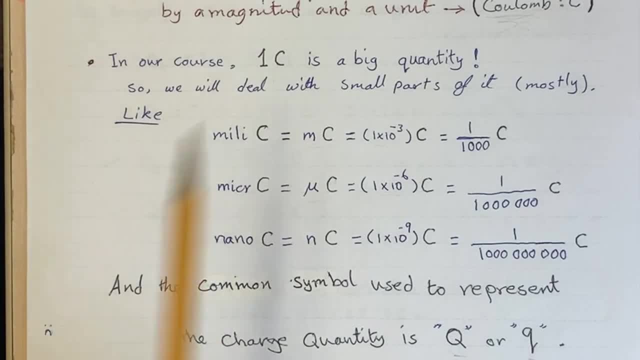 So in this course we are dealing with small quantities of that big quantity. So we will deal with milli Coulomb, which is 10 to negative 3 Coulomb or micro. this sample means micro Coulomb, which is 10 to negative 6,. 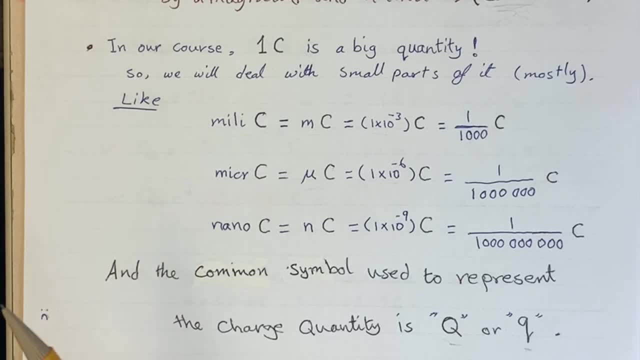 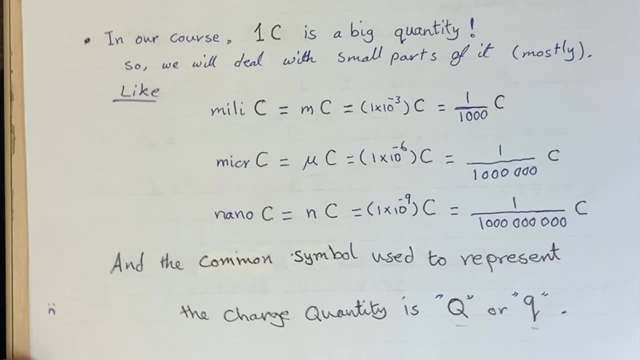 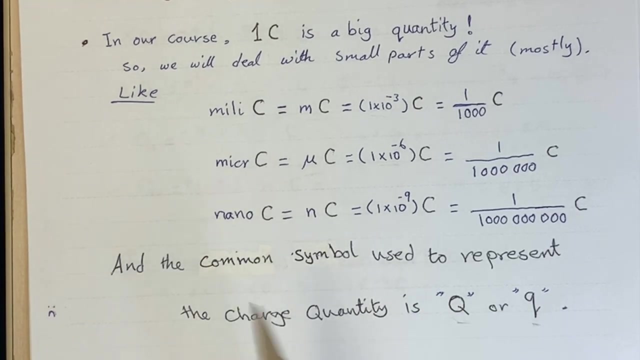 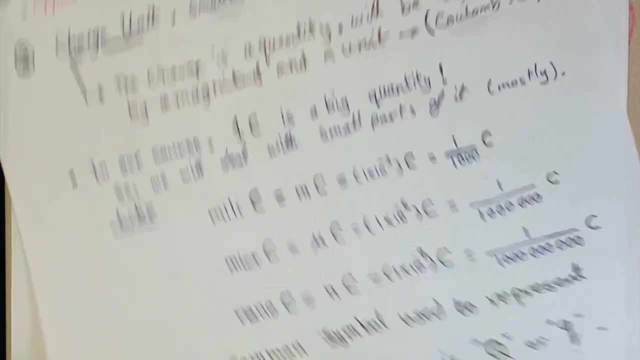 or one millionth, or nano, which is 10 to negative 9,, which is billionth of a Coulomb, And the common sample used in the solution for any problem is Q, which is in the higher case or lower case. So the sample of the charge quantity is Q. 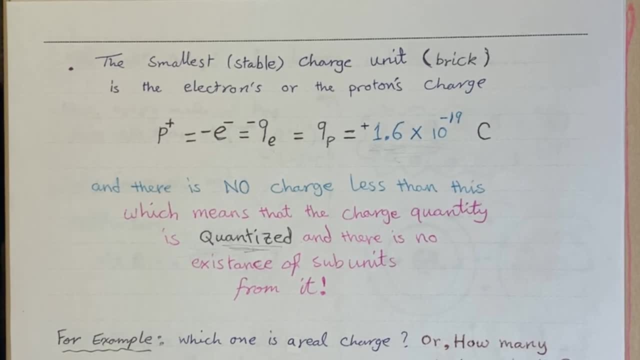 And the smallest charge, stable charge or the break to bolt. the other charge is the electron charge or the proton charge, which are the same, with negative sign which is equal to 1.6 multiplied by 10, to the negative 19 Coulomb. 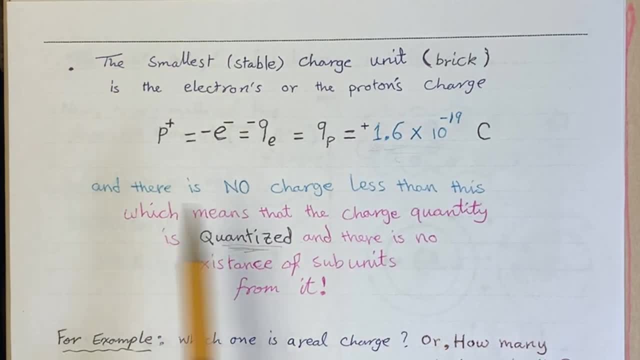 which is small quantity, The sample which what used for electron charge is E negative or QE, and the same for the proton QP or P plus. There is no smaller charge than this one. The electron is a particle, which is an elementary particle. 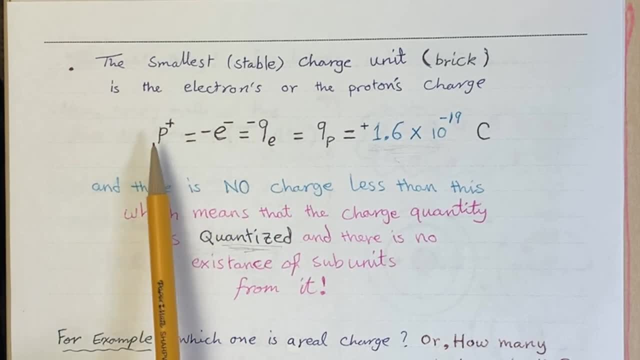 We cannot divide it to smaller pieces, But the proton, we can divide it to smaller pieces. actually, It is very stable. It is composed of other pieces and these pieces, some of them are with charge, third of this charge, or two thirds. 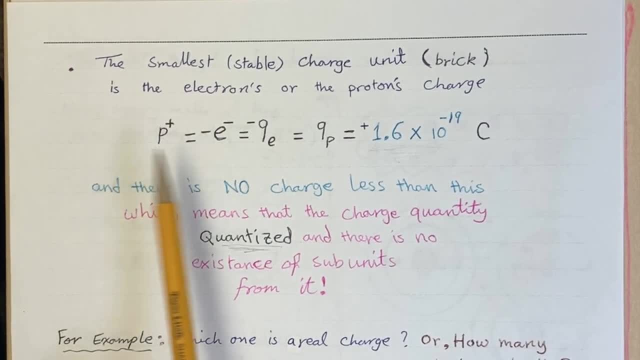 But these quantities, which are the quarks, they are not stable alone. They should compose another particle and the smallest charge according to that is the same charge which is 1.6 plus or minus times to the negative 19 Coulomb. 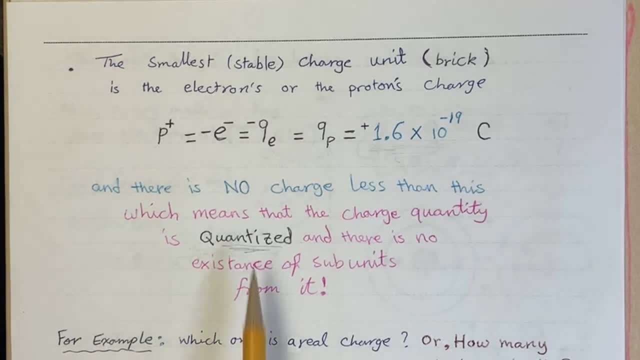 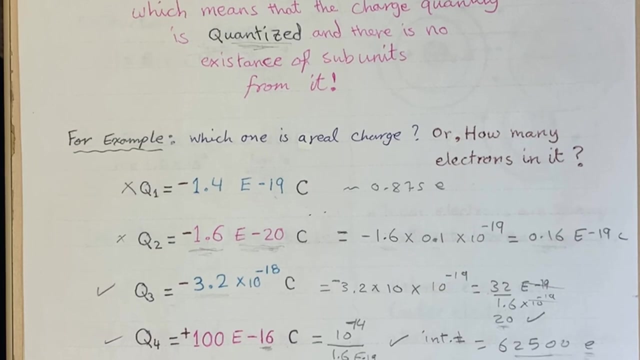 We mean by this? the charge is quantized. We have just integer number of charge. We don't have half or third of this charge quantity, which is the charge of electron. We can apply some example here with some quantities. I'm asking: 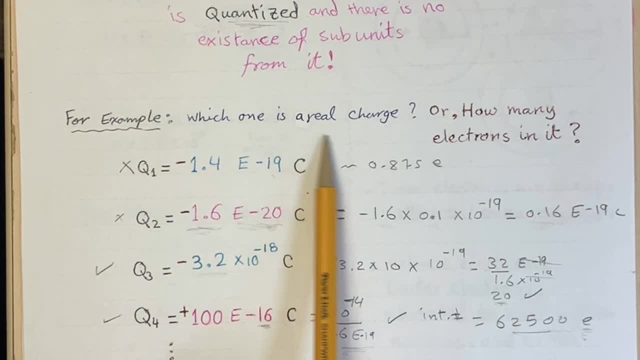 you can see this question: which one of them is real charge, or in different words, how many electrons or protons in this charge? We have Q1, which is the first charge, and I assume that this charge is negative 1.4, E, negative 19,. 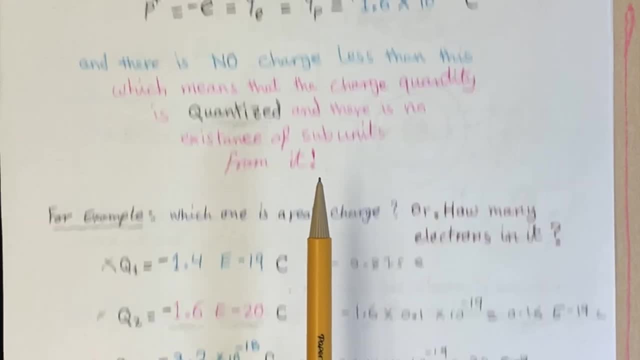 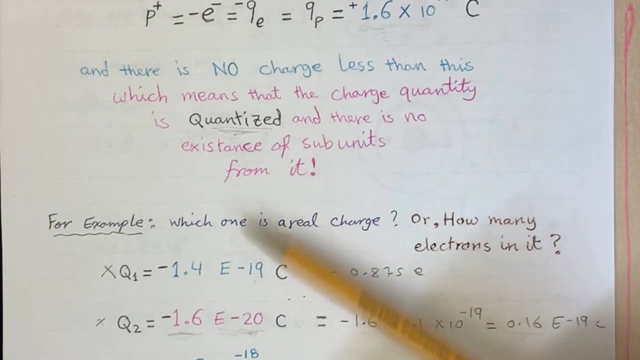 which is 10 to the negative 19.. Okay, The scale is 10 to the negative 19,, which is the same, But the charge here, as the electron I'm talking, 1.4- is smaller than the electron magnitude charge. 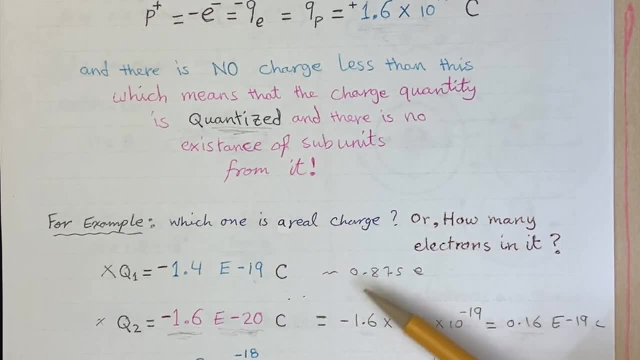 And if we divide 1.4 over 1.6, it's almost 0.875 of electron. We don't have any charge like this. Let us, for example, solve it for the second one, which is negative 1.6,. 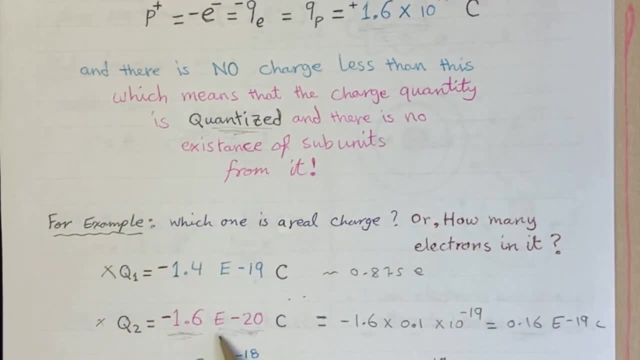 which is the same number, But now we have different. we have another thing which is important, which is the scale. Here we have 10 to the negative, 20,, 10 to the negative 19.. This, we convert this to this. 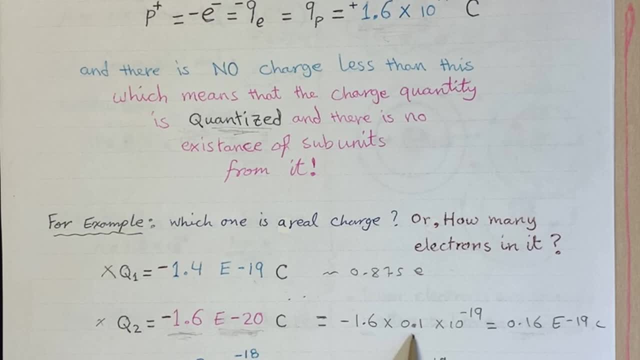 It's negative 1.6 times 0.1, 1 tenth times 10 to the 19 negative. So this make it 0.16, which is 1 tenth of the electron charge with the same scale. So we cannot find this charge. 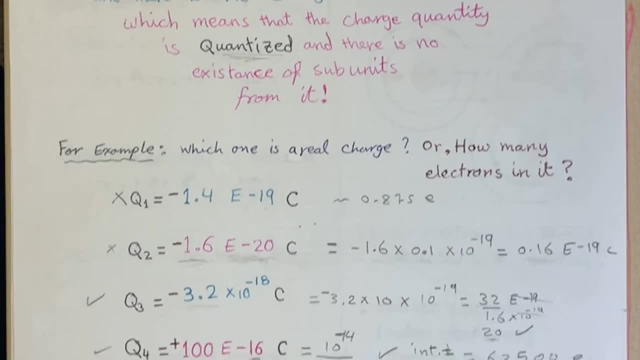 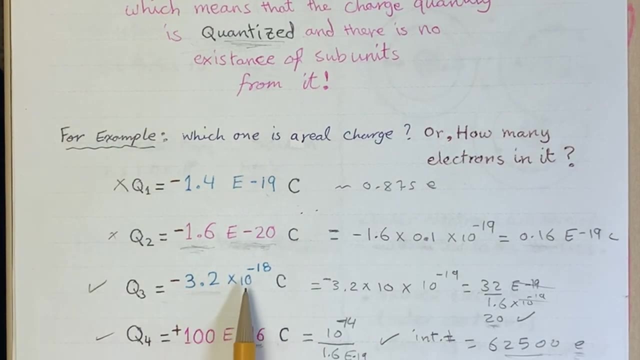 This is not a real charge. What about the third one? It's 3.2 with negative sign times, 10 to the negative 18.. 10 to the negative 18 is bigger than 10 to the negative, 19 by 10 times. 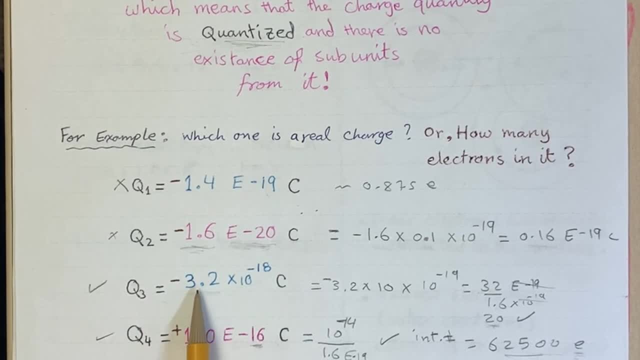 And we have negative 3.2.. Again, the sign is, for electron or proton, negative or positive. Now to put this as negative 10 to the negative 19, we will times multiply it by 10. So this charge equal to. 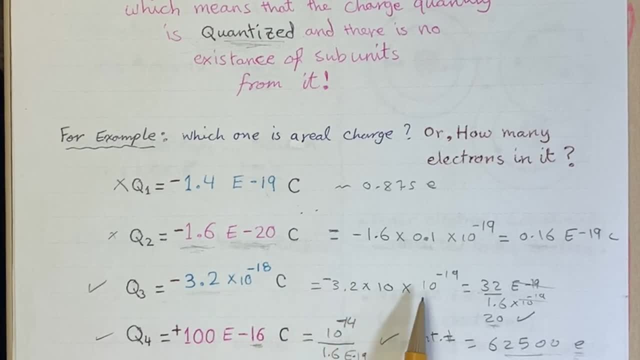 3.2 with negative sign times 10 to the negative 19.. This is equal to 32 times 10 to the negative 19.. And if we divide it by the charge of the electron, 1.6 times 10 to the negative 19, again. 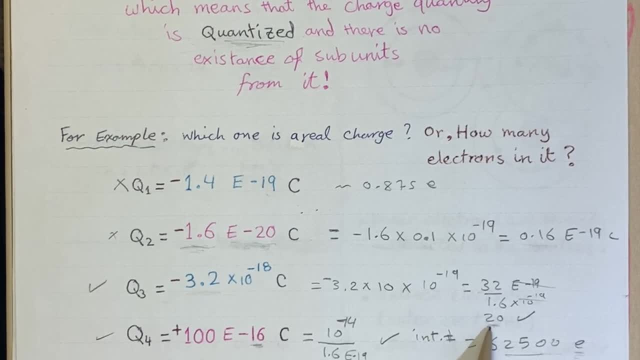 it will give us 20.. So we have 20, which is an integer number. Or we have 20 electrons composing this charge, So it's a real charge. What about this one? 100 times 10 to the negative 16,. 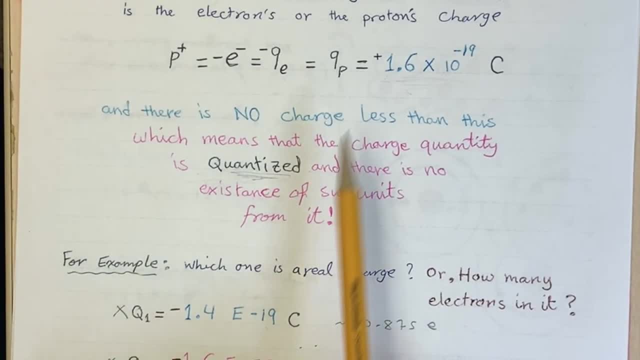 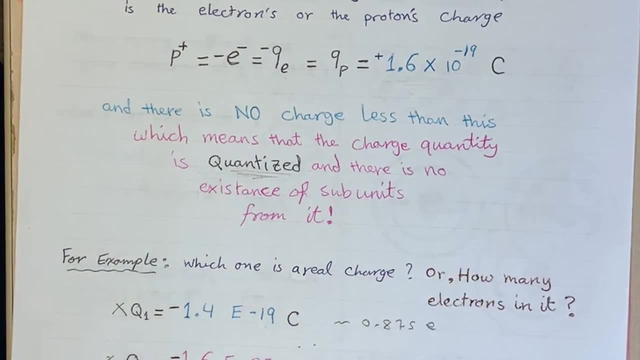 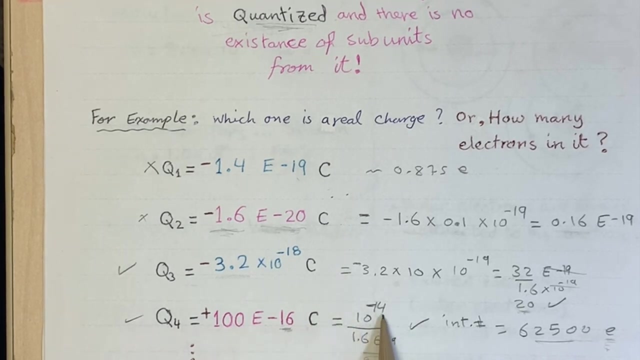 which is much bigger than negative 19. in this scale, 10 to the negative 16 is 1000 times bigger than this Time it, by multiply it by 100, make it 10 to the negative 14.. If you divide it on the charge magnitude, 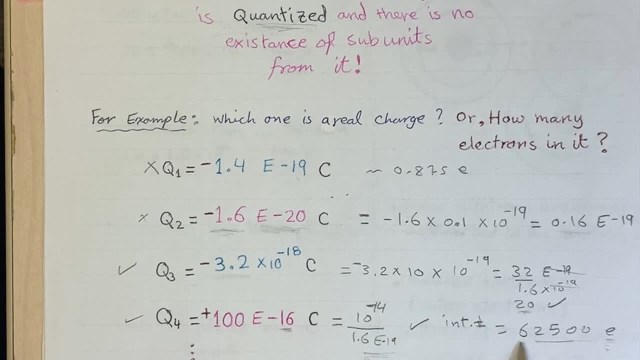 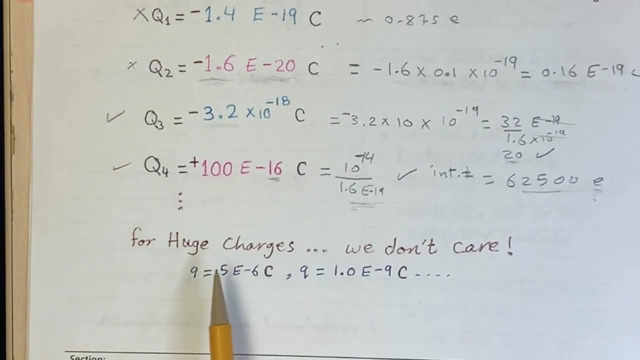 for the electron, it will give you an integer number, which is this one. So this is a real charge, Actually, for large or huge charge. what we get in this course, like micro or nano, we don't care about the quantization. 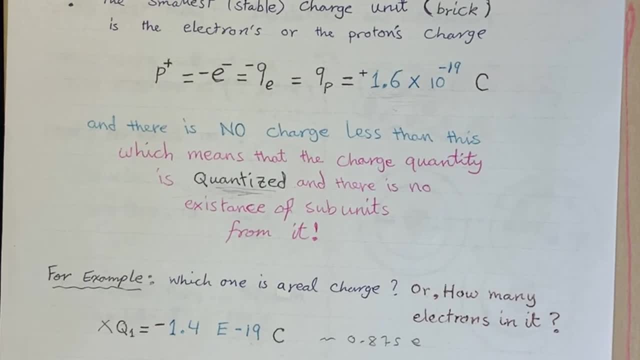 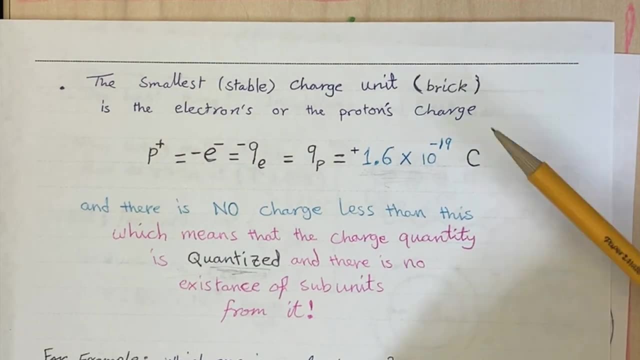 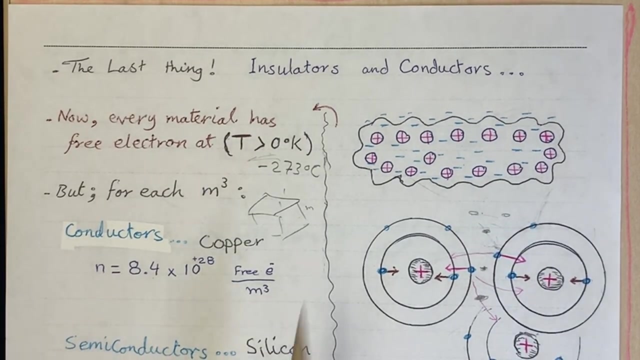 of the charge, because it is much bigger than what we considering that the electron charge is Now. finally, we need to discuss simple things about the insulators and conductors As we defined before, the atom components. we have the nuclei, we have electrons rotating around them. 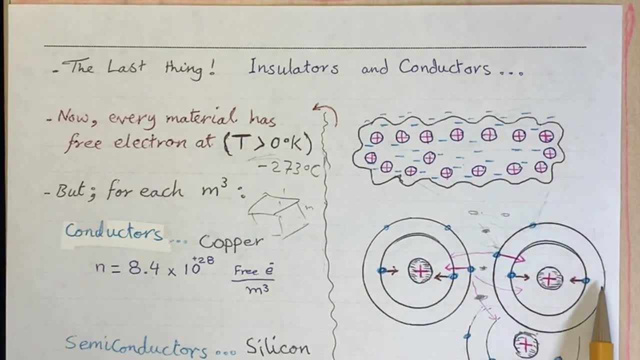 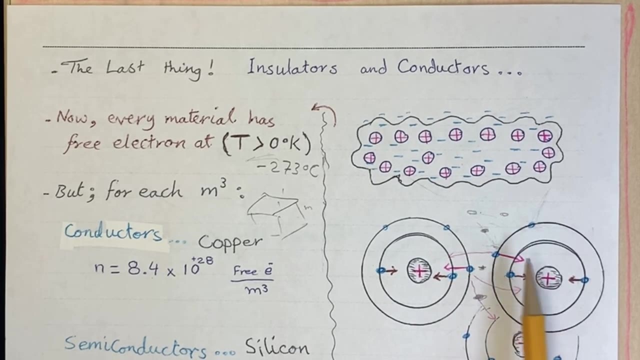 in the orbitals There are some electrons which are in the inner orbits. They are tightly or strongly attracted to their mother nucleus. They cannot escape, actually enter under any small forces. But for the outer electrons, if we give them some energy. 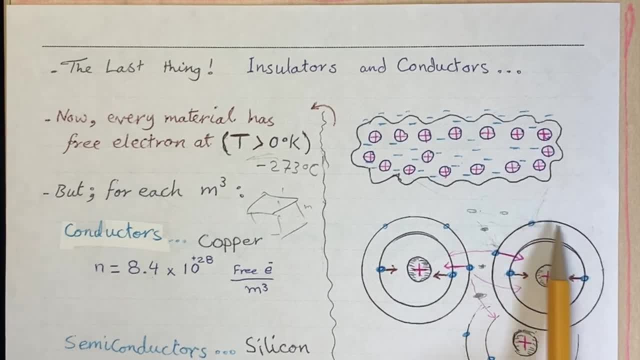 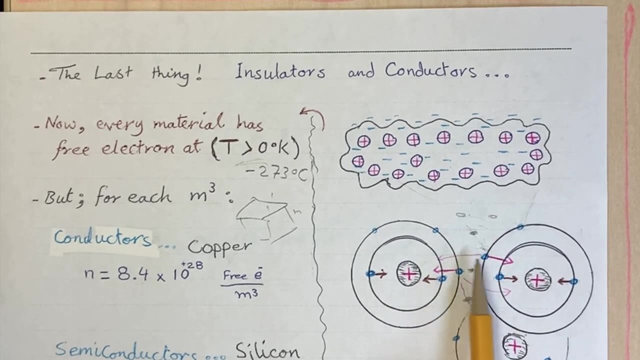 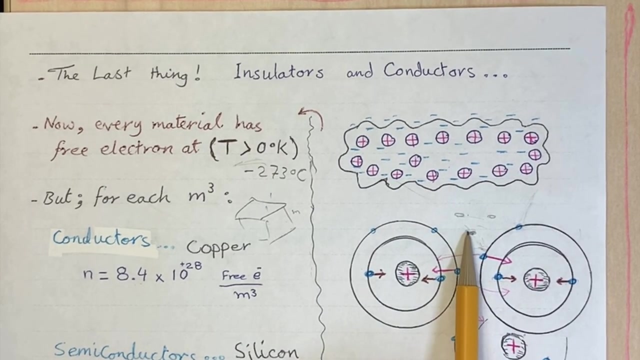 they are. they tend to escape, Especially if you know that there is another positive nucleus on the other side attracting them. This makes the escaping easier for them. Once they are outside, they are not belonging to any one of these atoms. They will be free electrons. 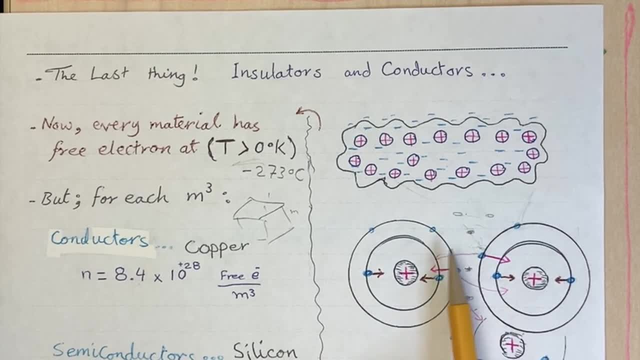 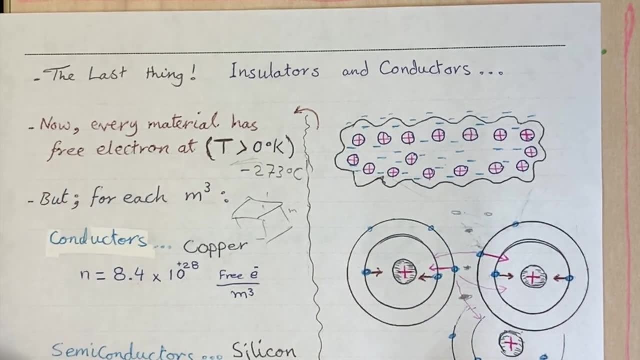 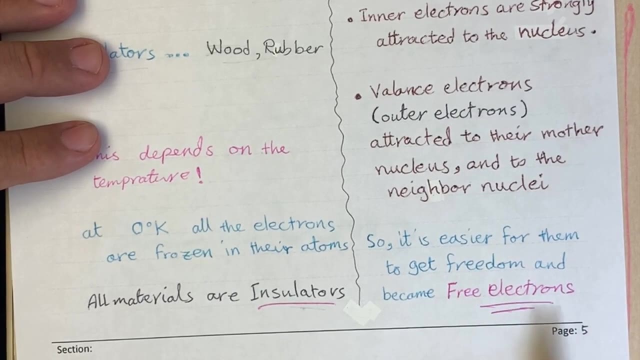 Maybe sometimes some atom capture them and keep them here temporarily, but they will escape again at that daily temperature, at high temperatures. But in general we will have in this material some free electrons, defined as free electrons, So the material composed of nuclei. 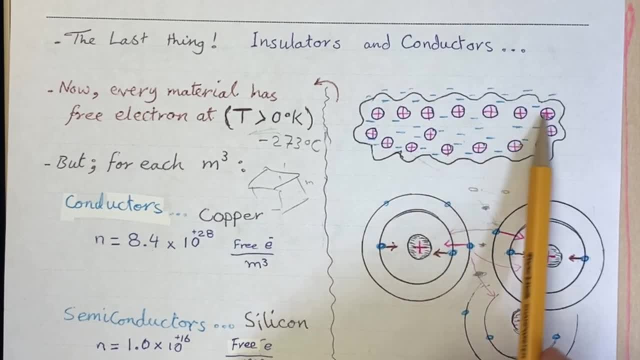 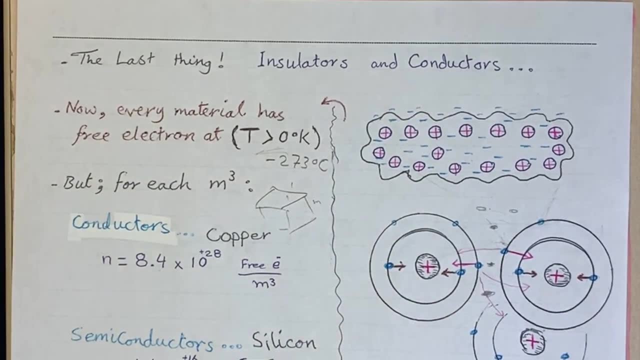 and some free electrons inside and on the surface of any material. Okay, To study this in physics quantitatively, we need to define things And we need to study, for example, some insulators or conductors or semiconductors. 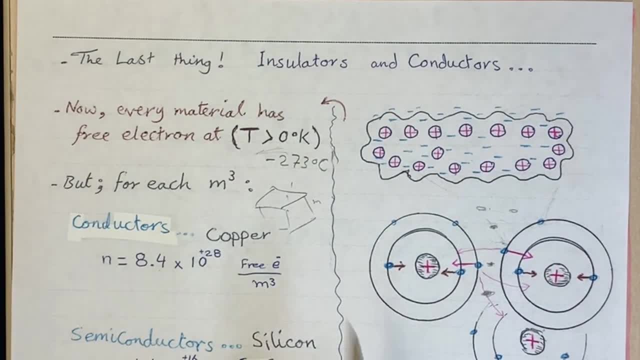 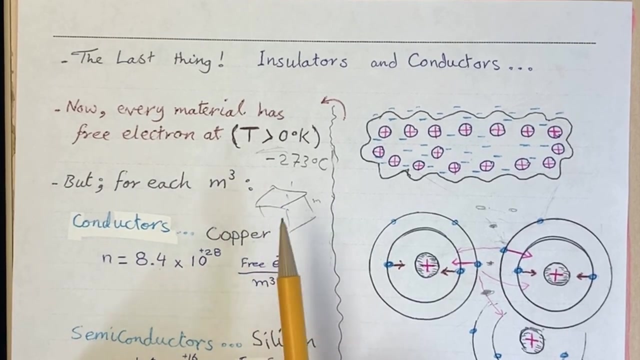 So we need to consider a volume for this. Consider one cubic meter of that material, For example the copper. In this one cubic meter we can count number of atoms according to the mass, the atomic mass of copper. We can count how many atoms here. 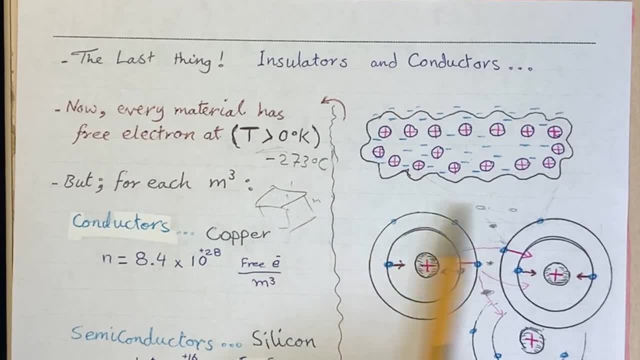 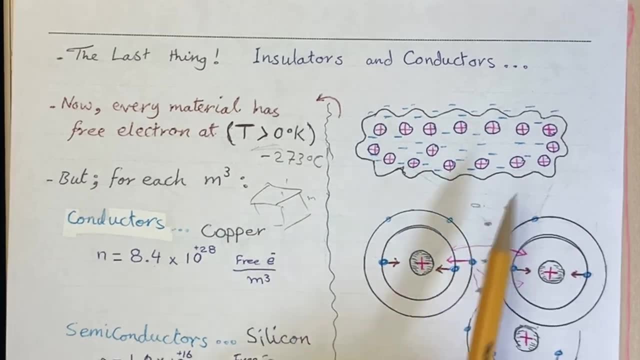 but we will not do that. Also, we can count the total number of protons or electrons or neutrons here, but we will not do that too. Also, we can count how many we have free electrons, but we will not do that. 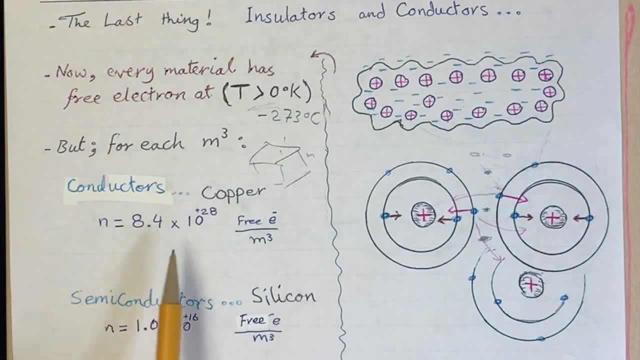 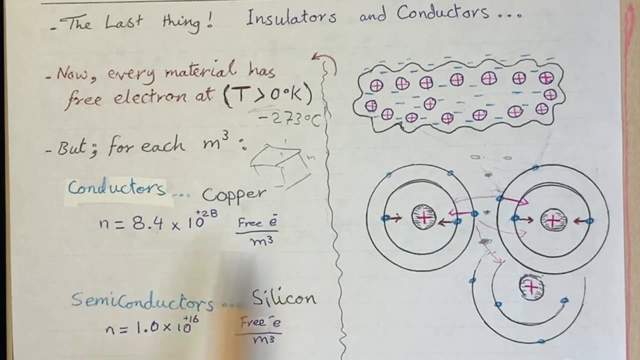 But I will mention just a number. For copper, for example, we have. number of free electrons inside one cubic meter equals to 8.4 times 10 to the positive 28.. Means we have 28 zeros. follows this number, which is very huge, huge number. 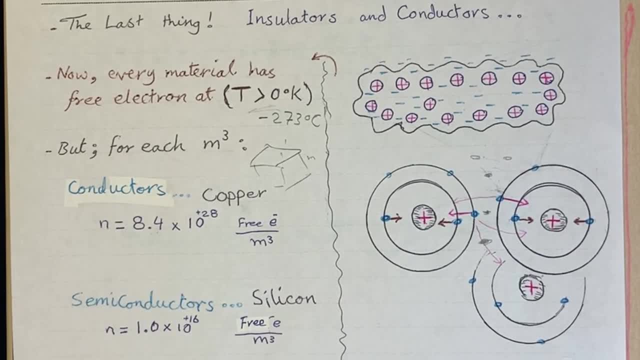 of free electrons inside one cubic meter. For silicon, which is a semiconductor like carbon, we have number times 10 to the positive 16.. It's a big number, but it is not huge number. So this material is semiconductor material. 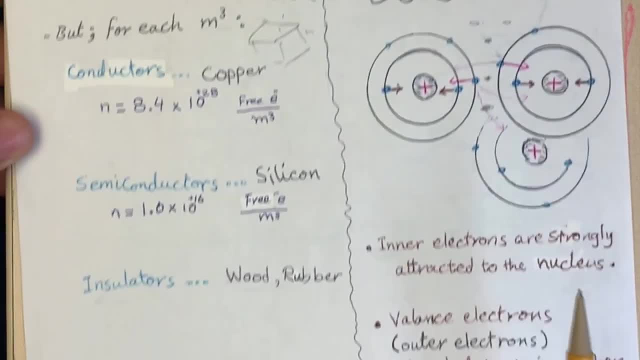 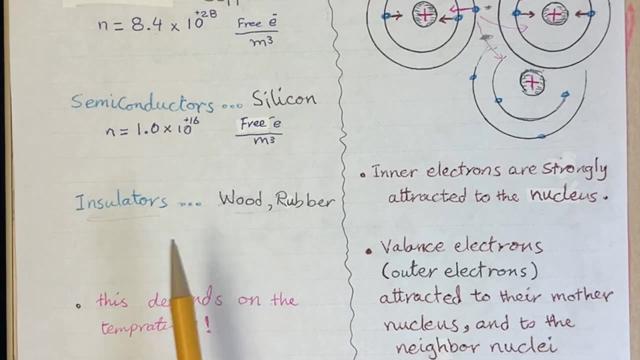 What do you think about insulators? If you look and Google that, you will find that they don't have any free electrons. That is not right or not exactly true. They have some free electrons, like thousands or millions, but they are much smaller than 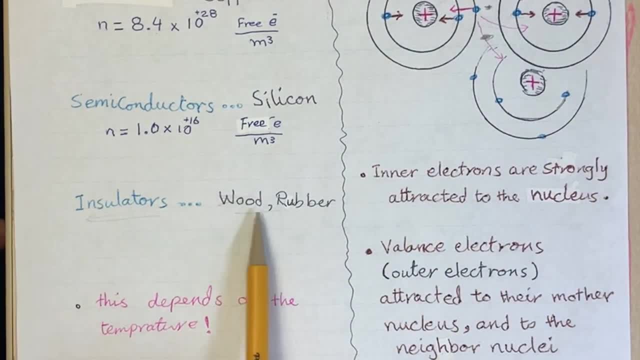 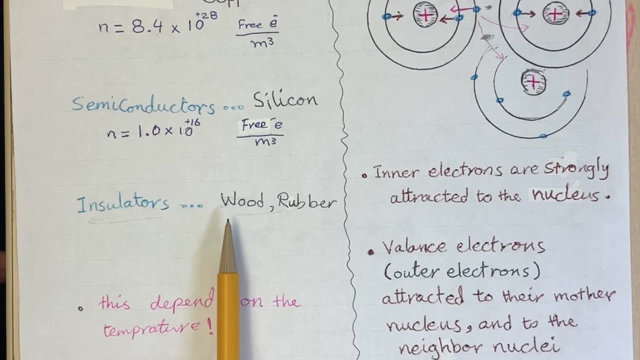 the semiconductors, for example. I'm talking here about dried wood. It doesn't have any humidity or water inside it, So there's no ions to carry the current or the charge from place to place. So for insulators we don't have any free electrons. 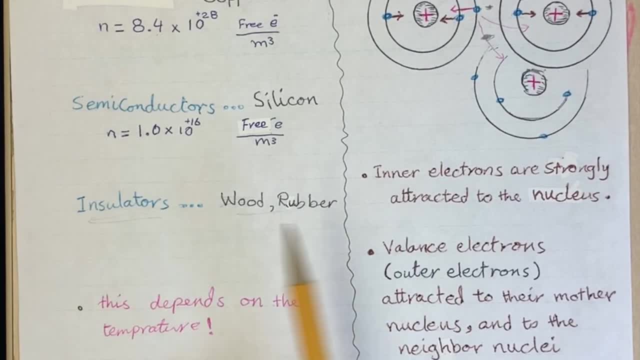 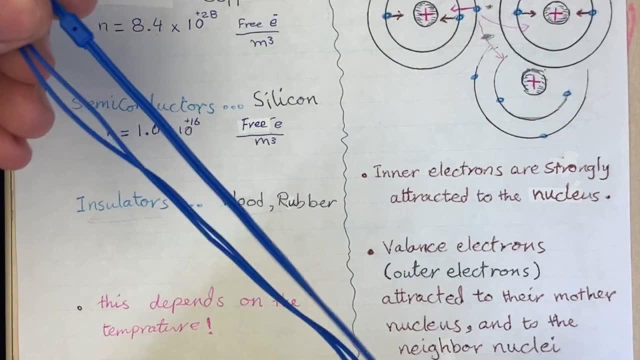 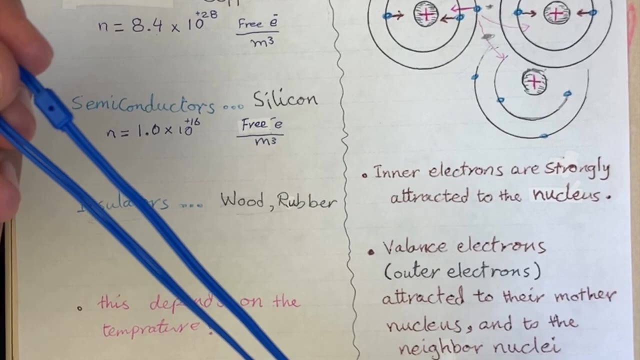 We can say this, but it is not accurate actually, because, for example, you know that we have wires, we have, we have plastic or rubber to insulate them, but some types of plastic is better than others, or rubber, So we have differentiation.